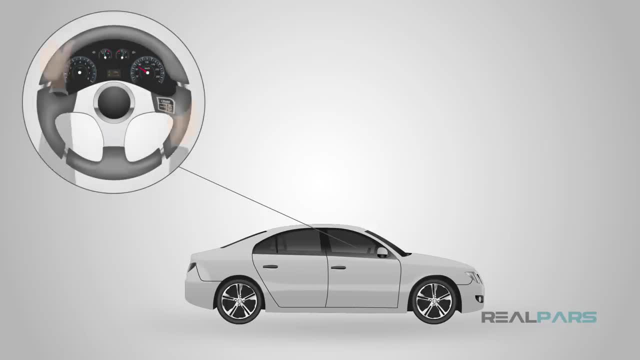 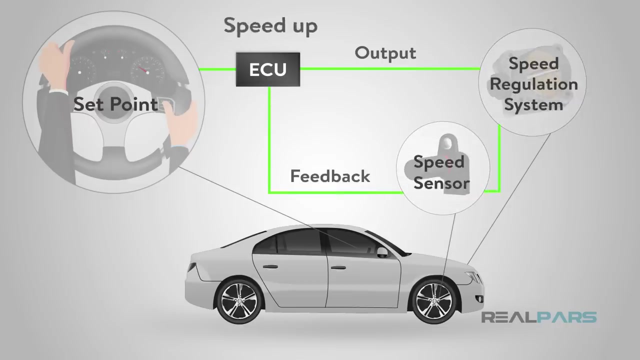 First you get to the speed that you want to be going. then you set your cruise control. The cruise control sends output signals to your throttle to regulate the speed. A speed sensor provides your control loop feedback. A speed sensor provides your control loop feedback to tell the cruise if the car should speed up or slow down. 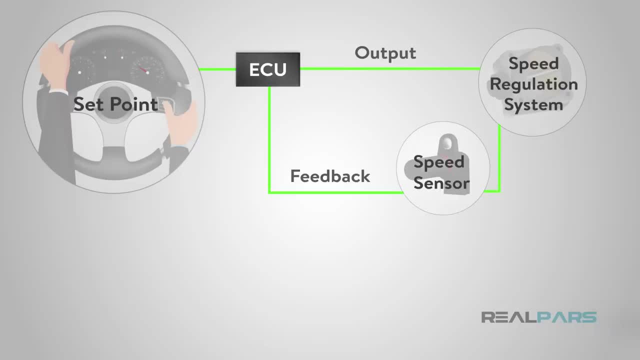 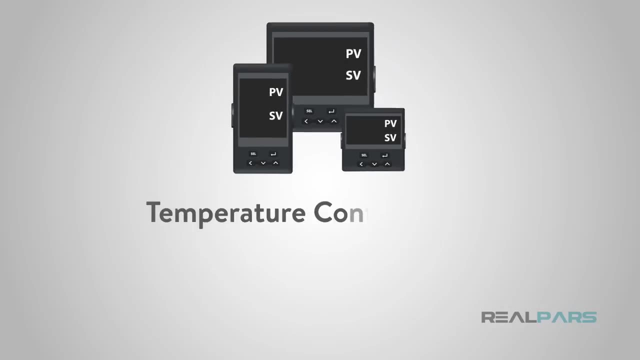 or how much more or less throttle to provide. A common standalone type that we use in manufacturing and industry is a temperature controller, PID. These controllers are pretty simple to use and set up. Plus, they do a great job at controlling temperatures of a variety of equipment. 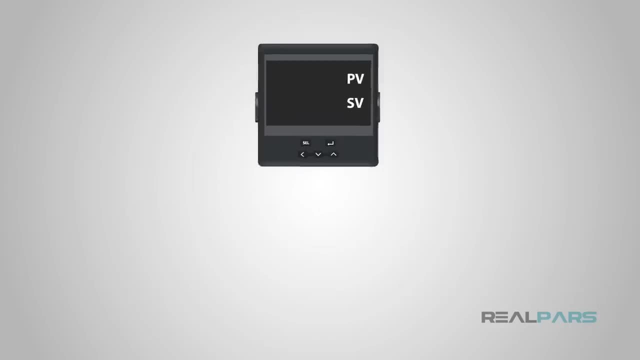 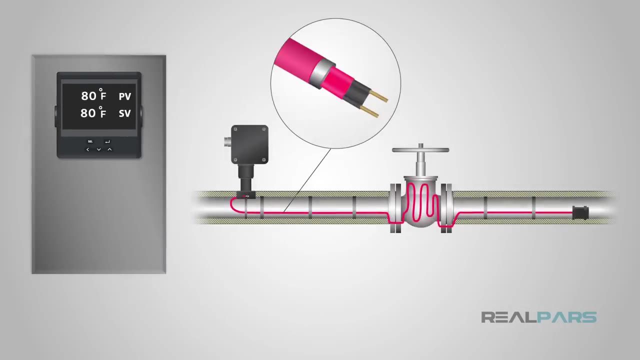 Let's take a look at how they work. For our example, we will look at a PID controller that controls the temperature of heat tracing on process piping. First we need to enter a setpoint- 200 degrees Fahrenheit, for our example. Now the controller will give a signal to the output to start heating up the heat tracing. 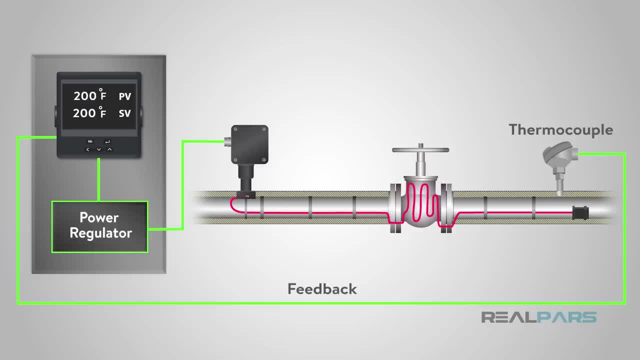 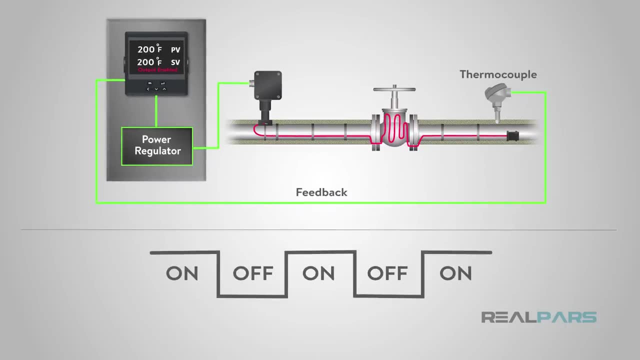 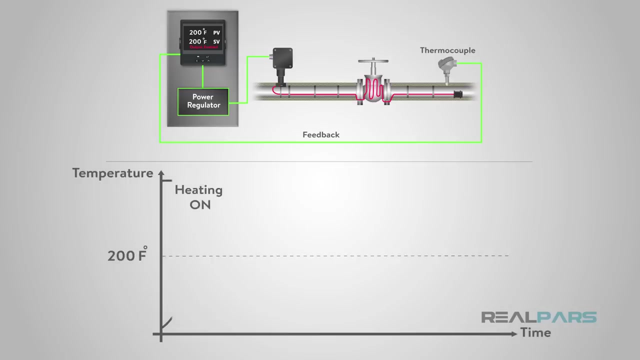 The control loop. feedback is in the form of a thermocouple to read the temperature. For our example, the PID controller can work as an on-off control for the heat tracing. Along with the setpoint of 200 degrees, we will set the controller at a couple of degrees above and below 200 as well. 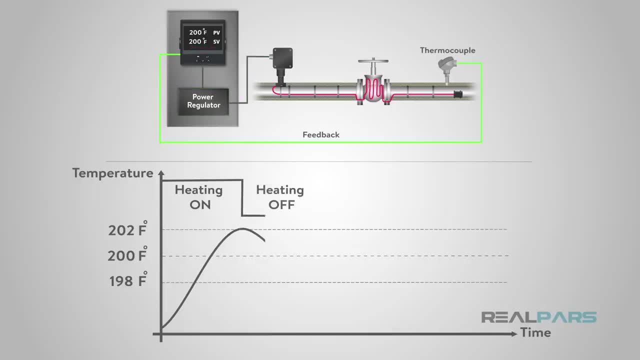 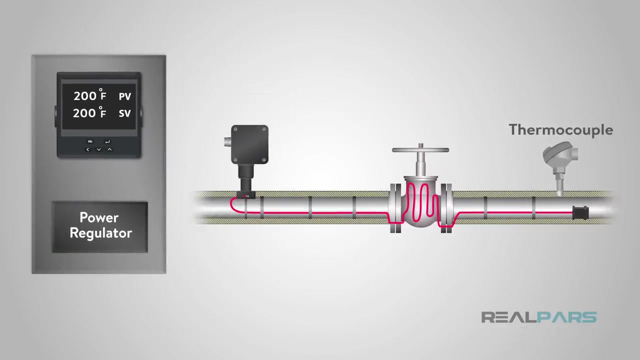 When the thermocouple reads 202 degrees, it will turn the heat tracing off. When it reads 198, it will turn it back on. This is the simplest form of PID control. We also have the option of setting up a PID controller with a PLC. 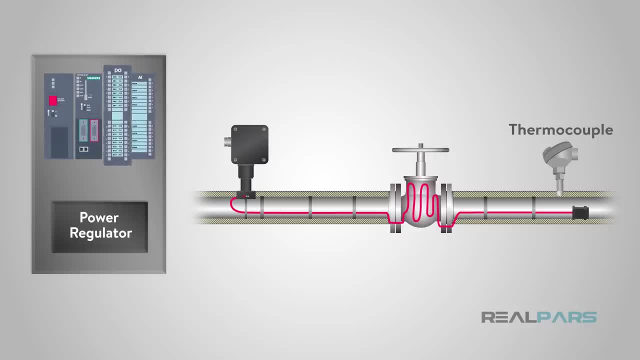 Instead of the standalone unit, we can use the input and output cards already on our PLC. The process variable or control loop feedback would be wired to our input card and programmed into the PID. Our output being controlled is wired to our output card. 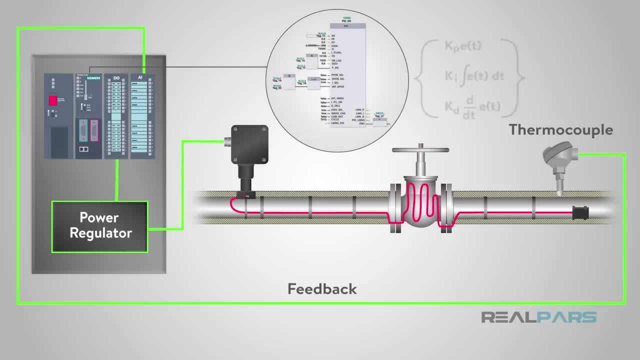 The PID and the PLC can do all of the math and make the decisions based on the variables and setpoints. No matter which way you decide to set it up, a PID is an excellent choice for an automated process. Let's look back at today's information.